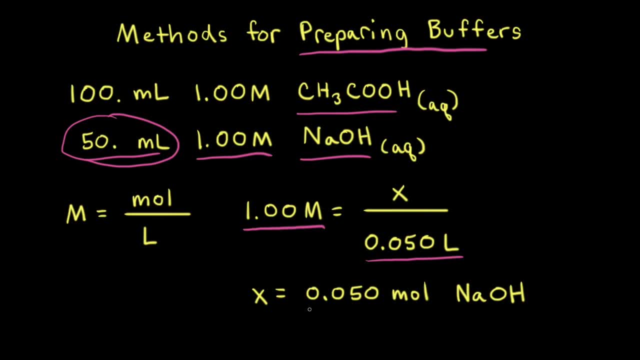 So, solving for X, we find that X is equal to 0.050 moles of sodium hydroxide. Since sodium hydroxide is a strong base, it dissociates completely in solution. Therefore, when we have 0.050 moles of sodium hydroxide, 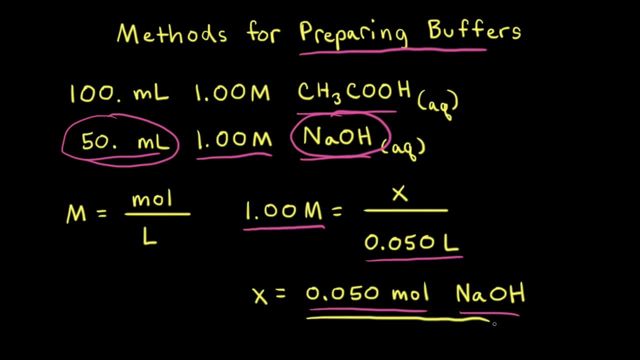 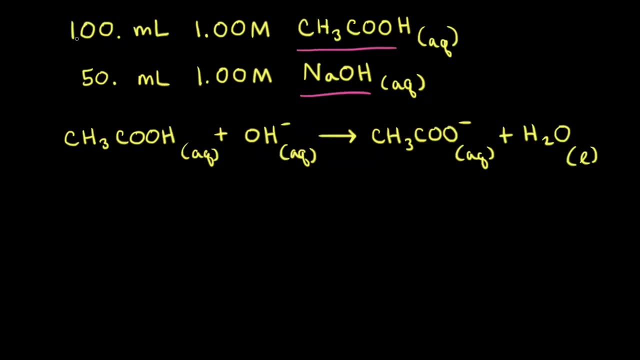 we also have 0.050 moles of sodium cations in solution and also hydroxide anions in solution. When these two aqueous solutions are mixed, we're mixing 100 milliliters with 50 milliliters for a total volume of 150 milliliters. 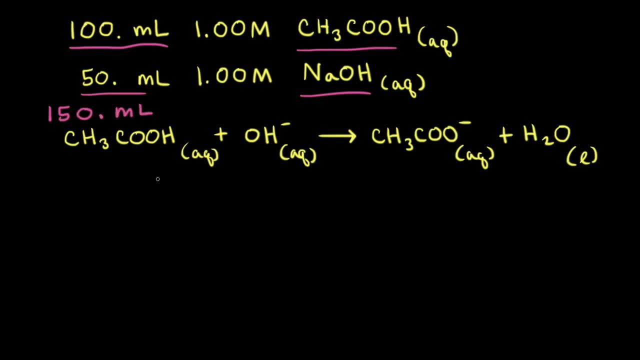 Let me just go ahead and write that down here really quickly. And when the two solutions are mixed, the acetic acid will react with hydroxide anions to form the acid, The acetate anion and water To figure out what's left over. 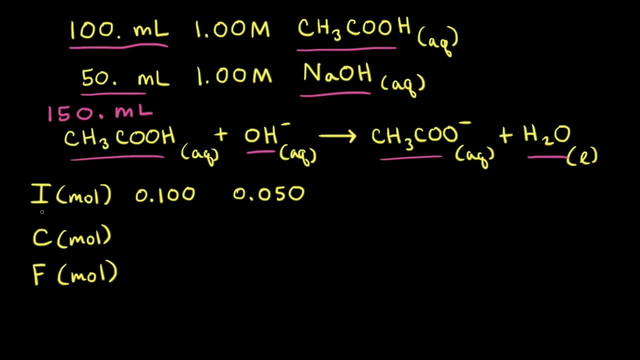 after the reaction goes to completion. we're gonna use an ICF table, where I stands for initial, C is for change and F is for final. We've already calculated. the initial number of moles of acetic acid is equal to 0.100. 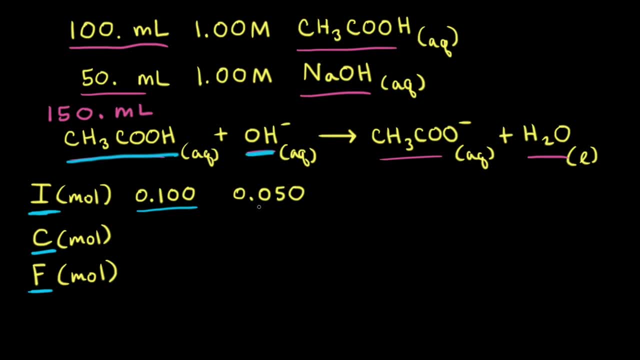 and the initial number of moles of hydroxide anions is equal to 0.050.. And if we assume the reaction hasn't happened yet, the initial number of moles of the acetate anion would be zero For this reaction. 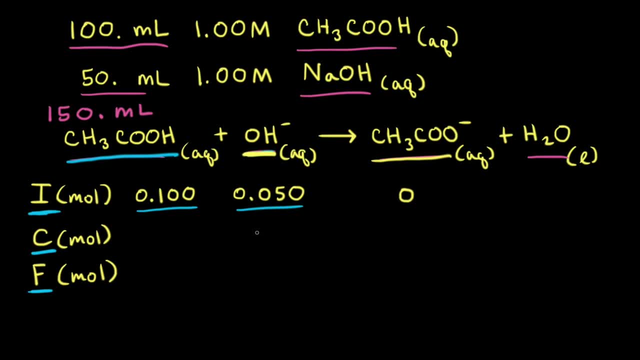 the hydroxide anion is the limiting reactant and therefore we're gonna use it all up in the reaction. So we write minus 0.050 under hydroxide in our ICF table. Looking at the balanced equation: the mole ratio of acetic acid to hydroxide anion. 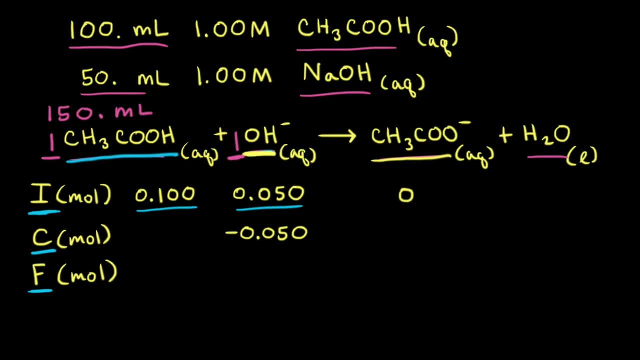 is one to one. Therefore, if we are losing 0.050 moles of hydroxide anions, we're also losing 0.050 moles of acetic acid. So when the reaction goes to completion, all of the hydroxide anions have been used up. 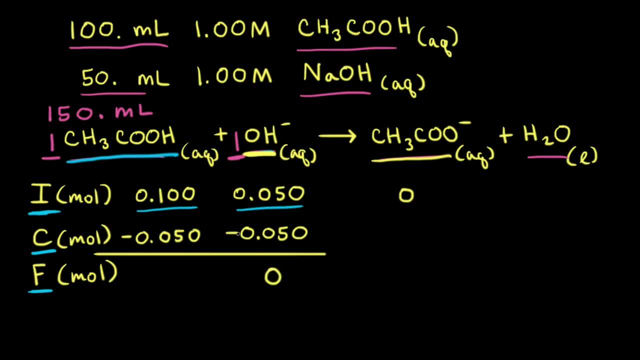 Therefore, we have zero moles of hydroxide anions leftover For acetic acid. if we started with 0.100 and we're losing 0.050, half of the acetic acid has been neutralized by the hydroxide anions. 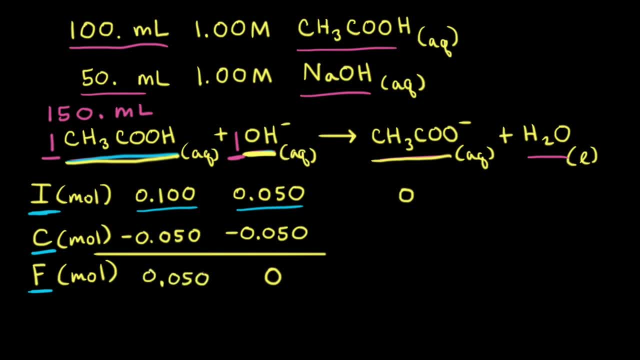 and we're left with 0.050 moles when the reaction goes to completion. For the acetate anion, the coefficient in the balanced equation is a one. Therefore, if we're losing 0.050 on the left side of the equation, 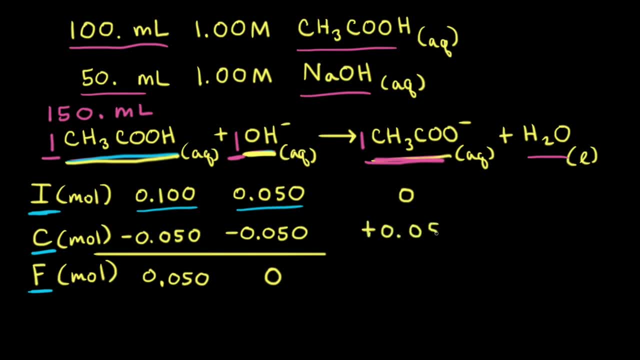 we're gonna be gaining 0.050 on the right side. So when the reaction goes to completion, we have 0.050 moles of the acetate anion. A buffer solution consists of significant amounts of a weak acid and its conjugate base. 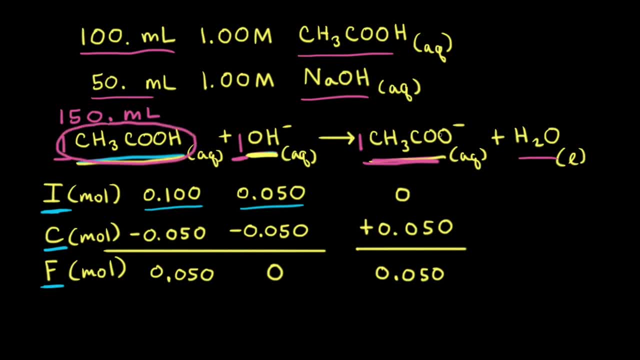 Acetic acid is a weak acid and its conjugate base is the acetate anion. Therefore, the addition of the strong base hydroxide, which neutralized half of the acetic acid, created a buffer solution, because we have significant amounts of both acetic acid. 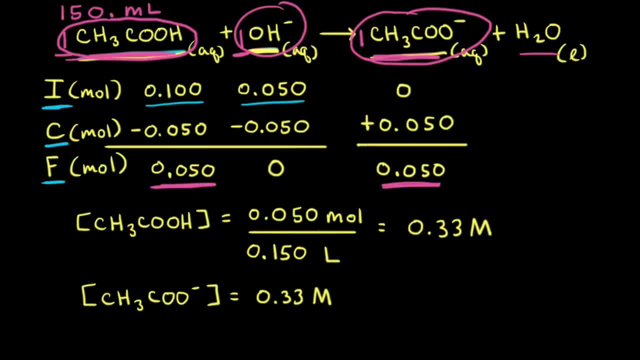 and its conjugate base, the acetate anion, in solution. Remember that our goal was to calculate the pH of this buffer solution. So first we need to calculate the concentration of acetic acid and of the acetate anion. To find the concentration of acetic acid. 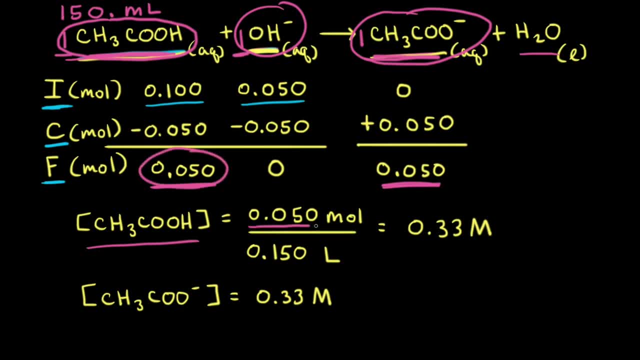 we take the moles of acetic acid, which is equal to 0.050, and we divide by the total volume of solution. We already calculated: when we mixed the two solutions together, the total volume was 150 milliliters, which is equal to 0.150 liters. 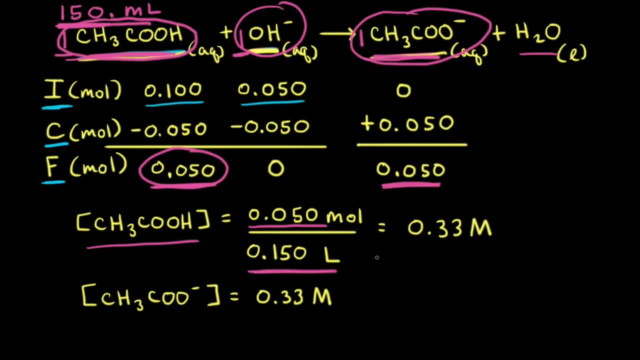 So 0.050 moles divided by 0.150 liters gives the concentration of acetic acid 0.33 molar. For the acetate anion we also have 0.050 moles and the total volume of solution is also 0.150 liters. 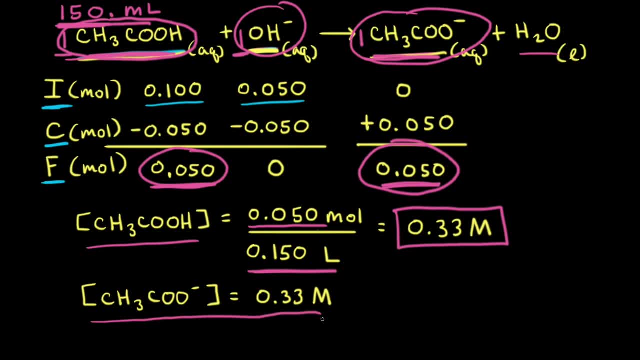 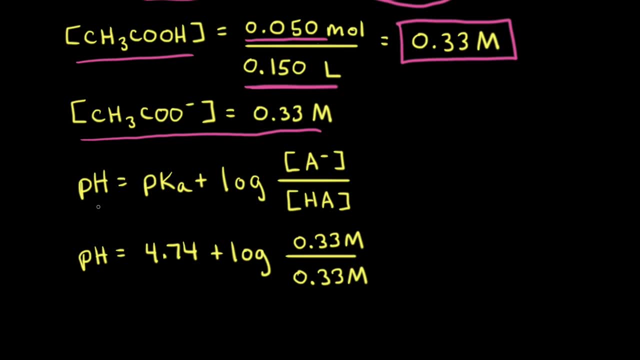 Therefore, the concentration of the acetate anion is also 0.33 molar. To find the pH of the buffer solution we can use the Henderson-Hasselbalch equation. The Henderson-Hasselbalch equation says the pH of the buffer solution. 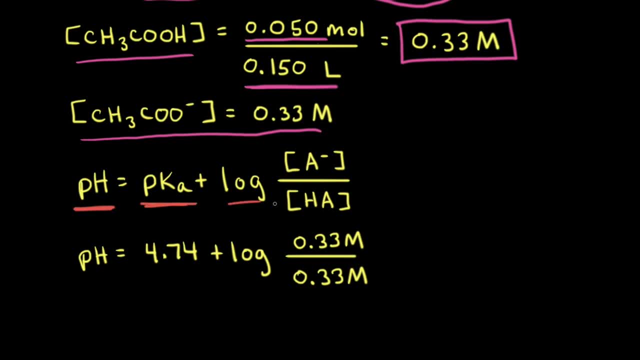 is equal to the pKa of the weak acid plus the log of the ratio of the concentration of the conjugate base divided by the concentration of the weak acid. The weak acid present in our buffer solution is acetic acid And at 25 degrees Celsius. 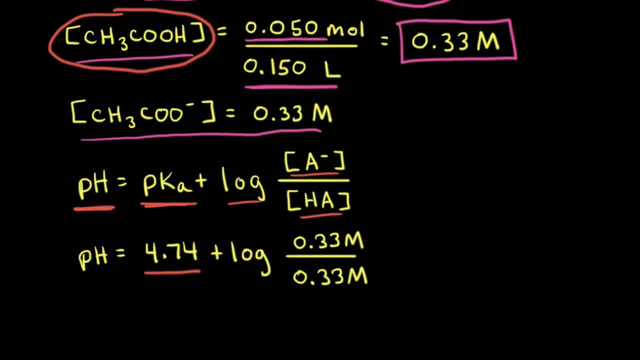 the pKa value of acetic acid is equal to 4.74.. The acetate anion is our conjugate base and it has the concentration of 0.33 molar, so we can plug that into the Henderson-Hasselbalch equation. 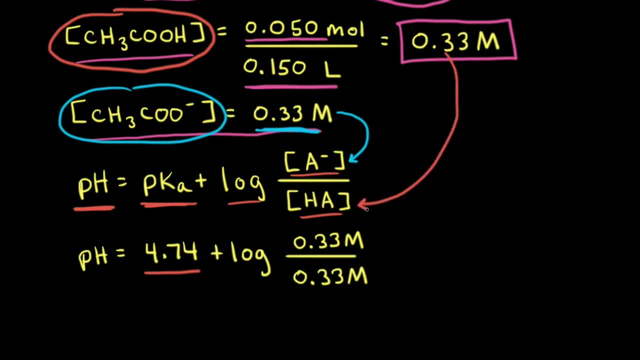 And the concentration of our weak acid is also 0.33. molar. Molar is canceled and 0.33 divided by 0.33 is equal to one And the log of one is equal to zero. Therefore, for this buffer solution, 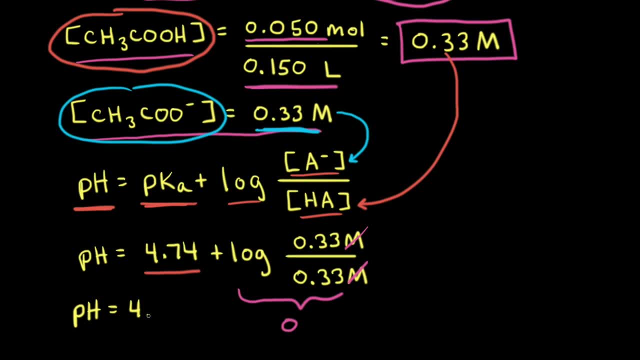 the pH is just equal to 4.74.. And notice that, even though I calculated the concentration of the weak acid and of the conjugate base, I didn't really have to if you look at the Henderson-Hasselbalch equation, because we have concentration divided by concentration. 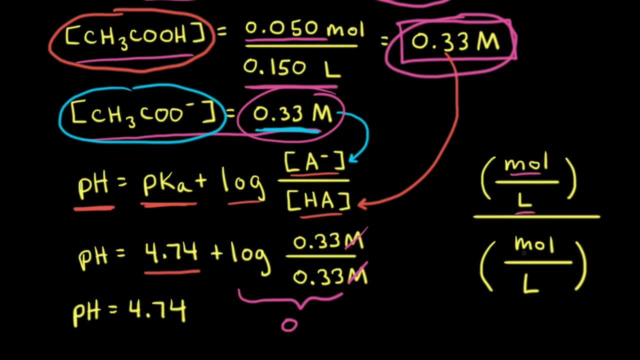 and concentration molarity is moles per liter, And so it's moles divided by liters divided by moles divided by liters. And since both the weak acid and the conjugate base have the same total volume of solution, the total volume of solution would cancel. 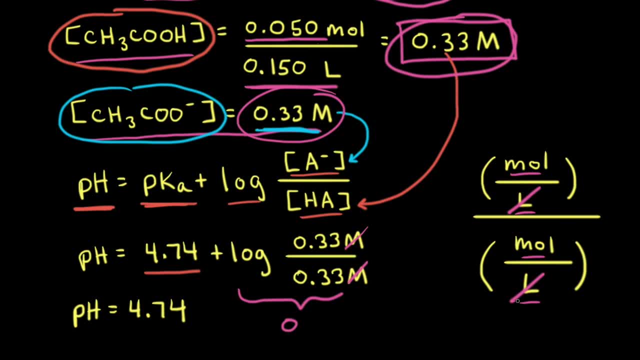 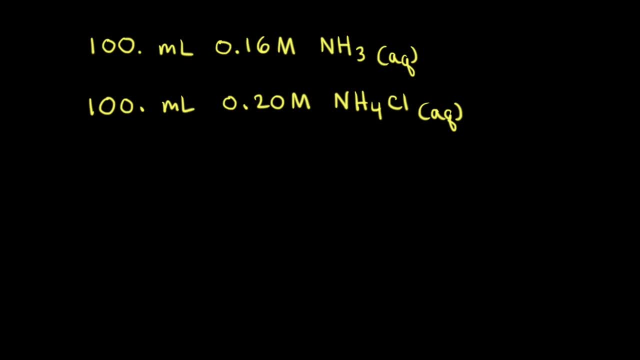 And so, if we want to, we could just do a ratio of the moles and we would have gotten the same answer: a final pH of 4.74.. Let's look at another method for making a buffer solution. In this case, we're gonna mix an aqueous solution. 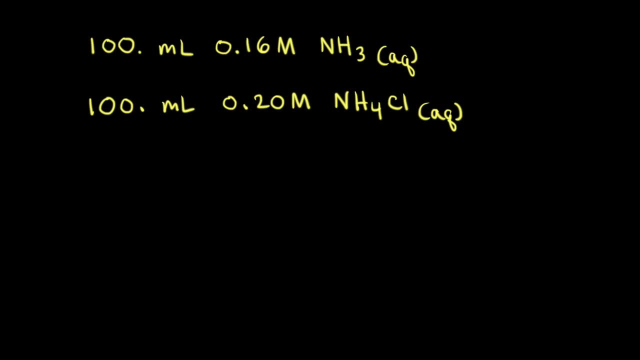 of a weak base with an aqueous solution that contains the conjugate acid to the weak base. In this example, our weak base is ammonia, NH3.. The conjugate acid to ammonia is the ammonium ion NH4 plus, And if we have an aqueous solution of ammonium chloride. 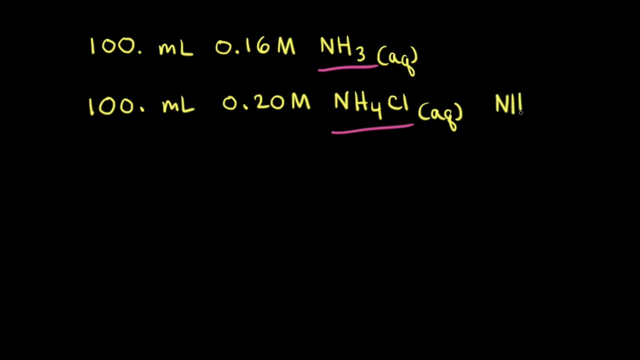 in solution there are ammonium ions, NH4 plus, So we have a weak base- NH3, and its conjugate acid, NH4 plus, And when the two aqueous solutions are mixed, we'll have a significant amount of both our weak base. 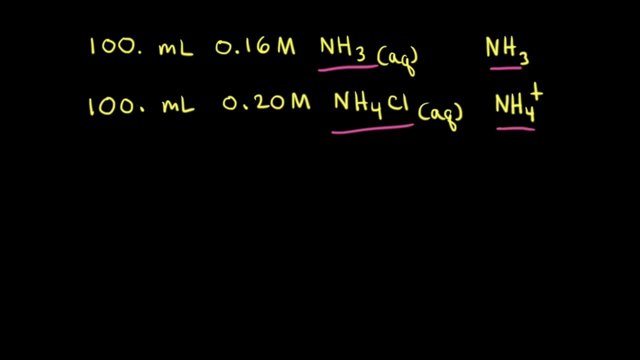 and its conjugate acid. Therefore, we will have a buffer solution. I often say that a buffer solution consists of a weak acid and its conjugate base. In this case, I've said, the buffer solution consists of a weak base and its conjugate acid. 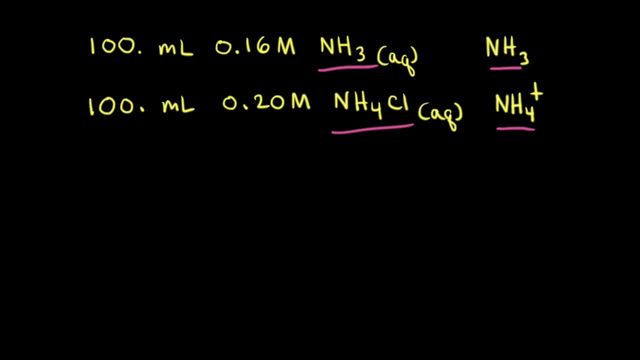 So a more general definition for a buffer solution could be a weak conjugate acid and its conjugate acid base pair. We can calculate the pH of the buffer solution that forms when we mix the two solutions together using the Henderson-Hasselbalch equation. 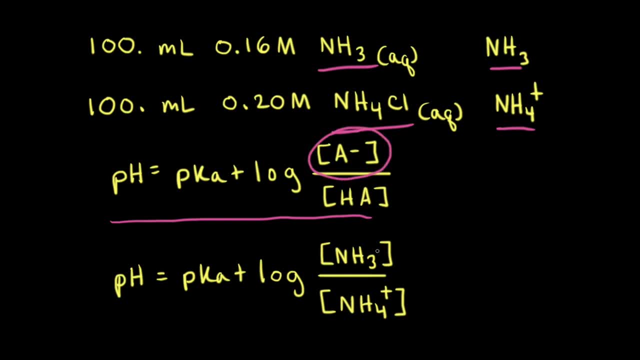 In this case, our numerator is our weak base, which is ammonia, and our denominator is the conjugate acid to ammonia, which is the ammonium ion NH4 plus The ammonia solution had a concentration of 0.16 molar. 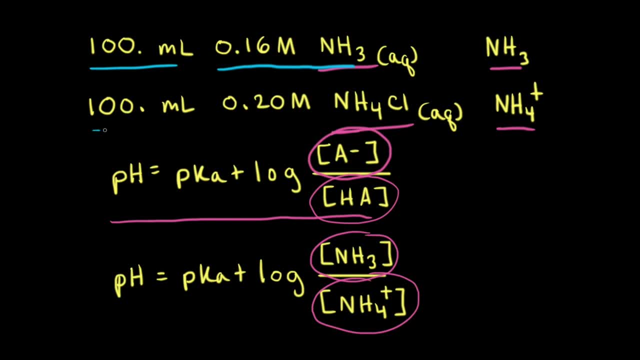 And when we mix 100 milliliters of the ammonia solution with 100 milliliters of the solution, we get a concentration of 0.16 molar. And when we mix 100 milliliters of the ammonia solution with 100 milliliters of the solution, 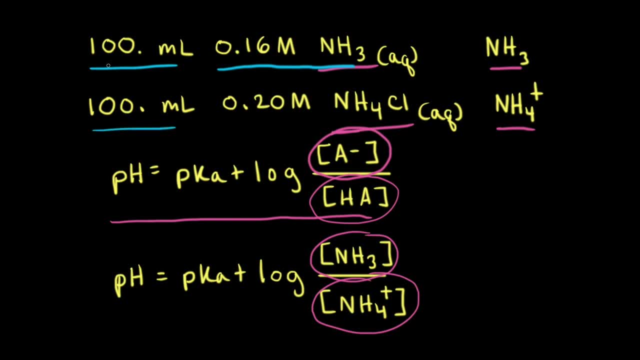 of ammonium chloride, the total volume would double. So we went from 100 milliliters to 200 milliliters. Therefore, since we're doubling the volume, we're having the concentration of ammonia, So we can put in 0.080 molar. for the concentration of ammonia. Ammonium chloride is a soluble salt. Therefore, if we have 0.20 molar for the initial concentration of ammonium chloride, we have 0.20 molar for the initial concentration of ammonium ion. 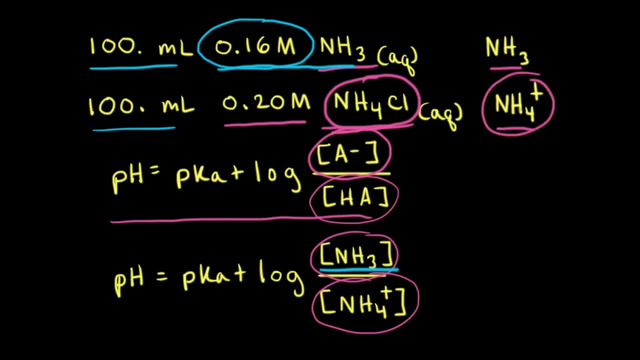 And since we're doubling the volume when we mix the two solutions together, we are having the concentration. So the concentration of ammonium ions in solution is 0.10 molar. So we could plug that into the Henderson-Hasselbalch equation. 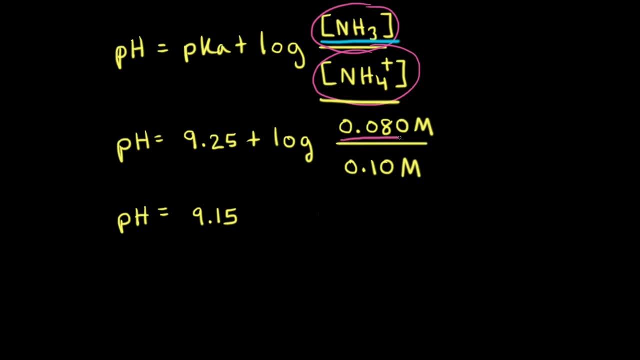 So here we have the concentrations plugged in: 0.080 molar is the concentration of ammonia and 0.10 molar was the concentration of the ammonium ion. In the Henderson-Hasselbalch equation, the pKa is the pKa of the ammonium ion. 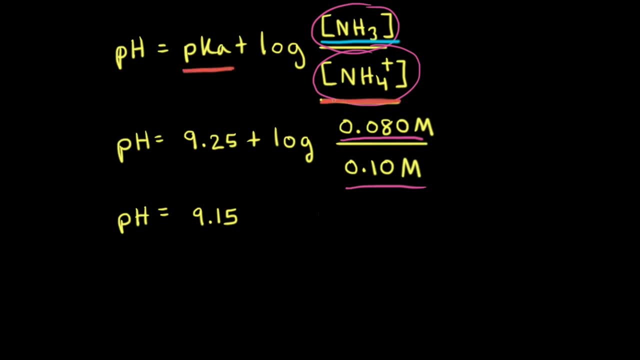 The pKa value of the weak acid, which is the ammonium ion, NH4 plus. At 25 degrees Celsius, the pKa value of the ammonium cation is equal to 9.25.. Molar cancels and when we solve for the pH of the solution. 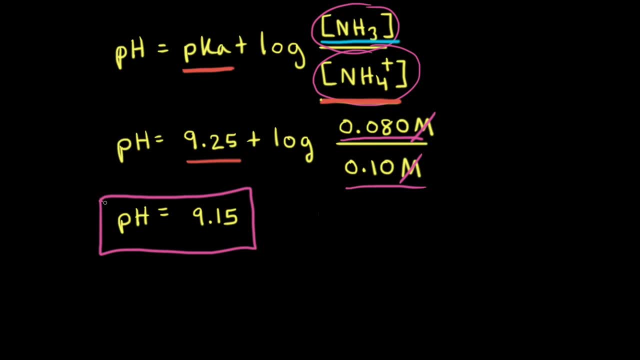 the pH is equal to 9.15.. So this problem started with a weak base and a salt that contained the conjugate acid. to that weak base. It's also possible to make a buffer solution, starting with an aqueous solution of a weak acid.